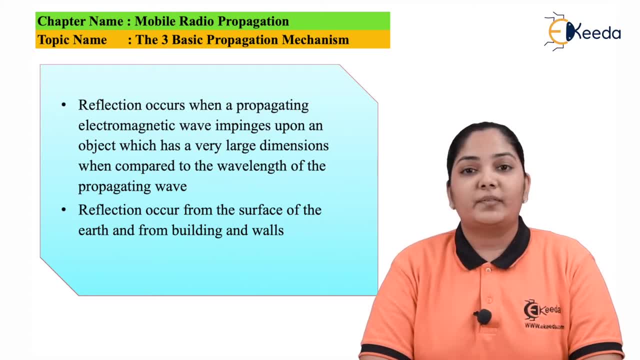 There are many such obstructions or objects through which the reflection takes place. For example, consider buildings, trees, etc. These are the places through which the reflection will take place and reach the receiver. The biggest path through which the reflection takes place is nothing but the ground or the earth's surface, Whenever the electromagnet 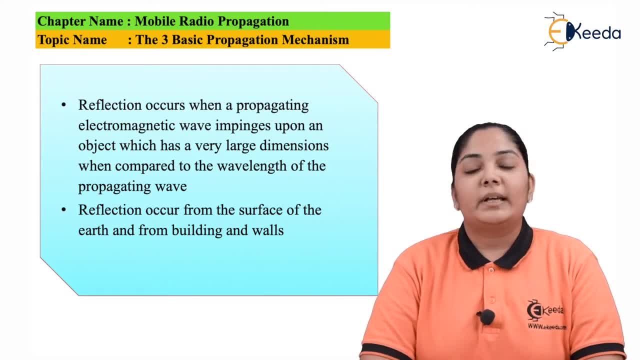 waves are traveling in multiple paths. there is one wave that gets reflected through this ground wave and then reaches the receiver, So there are various other parameters or objects available through which reflection takes place. Hence, reflection is one of the important parameter or important method through which the mobile radio propagation takes place. 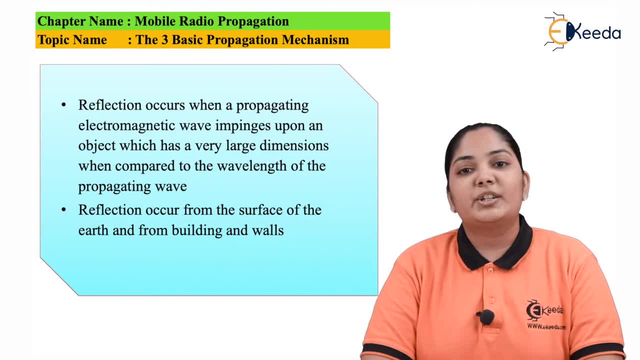 That is, the radio waves from the mobile transmitter reaches to the receiver. Let us now move towards the next method, that is called as diffraction. Diffraction is a function of radio waves. The wave is a symbol of the transmission of radio waves. The wave- 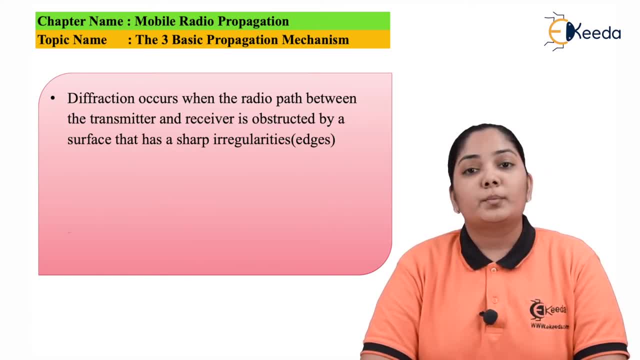 Diffraction occurs when the radio waves that are propagating are obstructed by sharp edges. This is called as diffraction. When they are obstructed by these sharp edges, there are secondary waves that are formed and these waves travel in all the directions. In other words, there 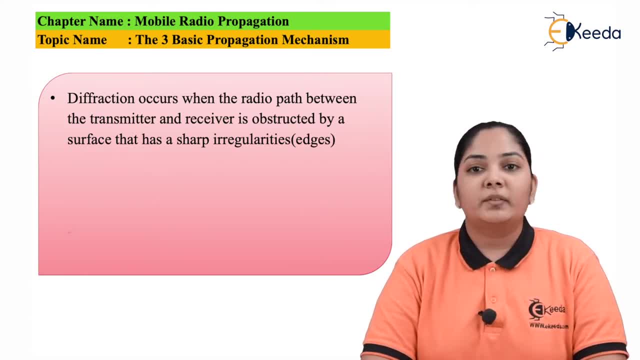 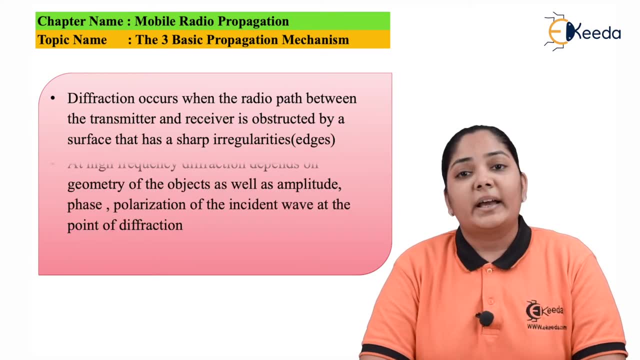 is a bending of the wave that takes place and diffraction is one of the reasons why we are getting our radio waves or why we are able to receive the electromagnetic mobile transmission At higher frequencies. the diffraction depends upon the objects, that is, the geometry of the object. 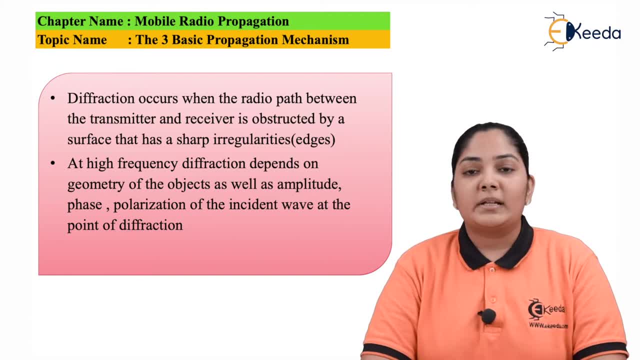 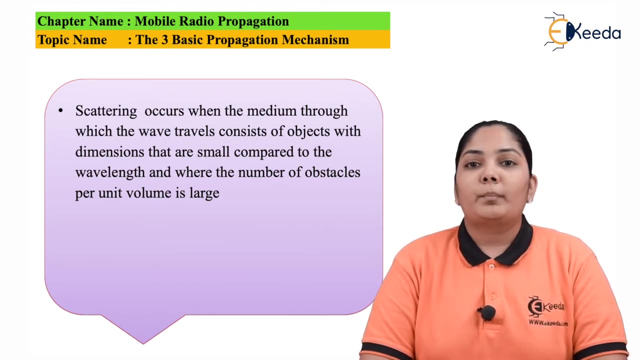 the amplitude and other parameters. It also depends on the phase and the polarization of the electromagnetic waves as well. Let us now move towards the last parameter, or the last method through which the radio propagates, that is called as scattering. So in scattering the electromagnetic 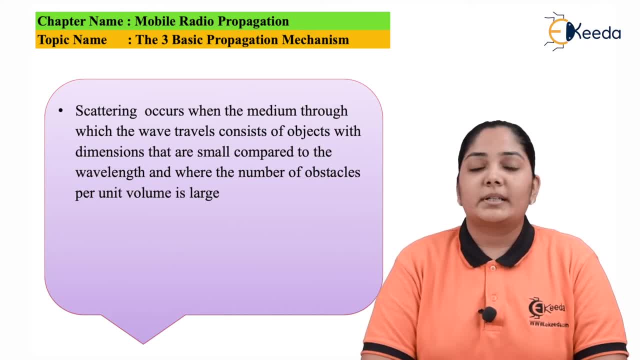 waves that are propagating are obstructed by objects that are very small with respect to the wave. So, in scattering, the electromagnetic waves that are propagating are obstructed by objects. wavelength of the communication. Wavelength, as we all know, is the parameter through which the 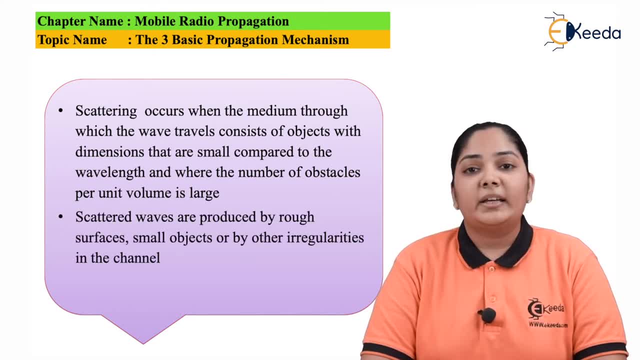 frequency is decided. So example: if we take higher frequency, that is, of 10 gigahertz, then the wavelength will be in terms of millimeters. Hence, as the radio is moving through the channel, there are various objects of the length of millimeter or less than the wavelength, and hence the scattering.